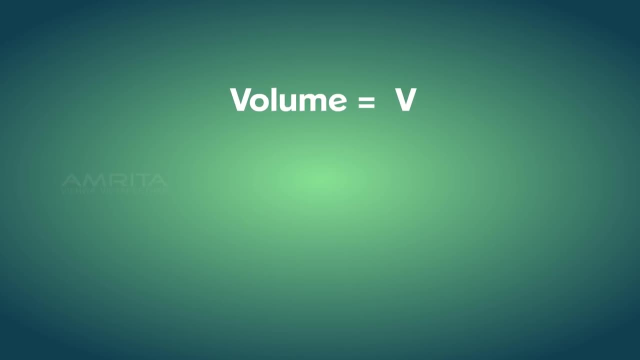 of the buoyant force depends on the volume V of the immersed part of the body, the density rho of the fluid and the acceleration of the buoyant force. In general, an object experiences a loss of weight in water due to the upthrust and it. 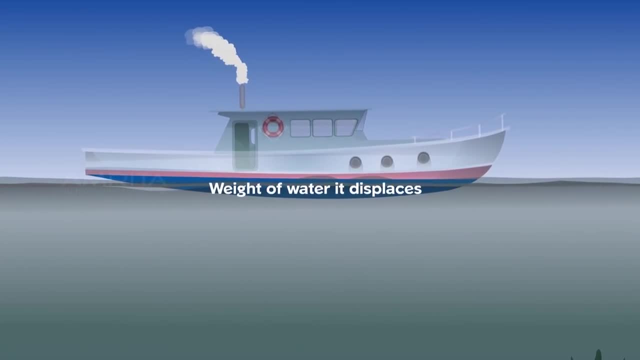 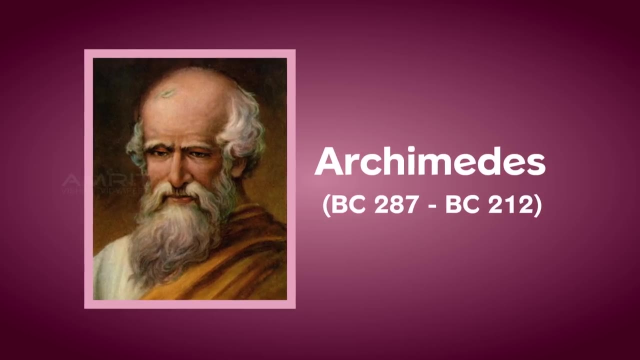 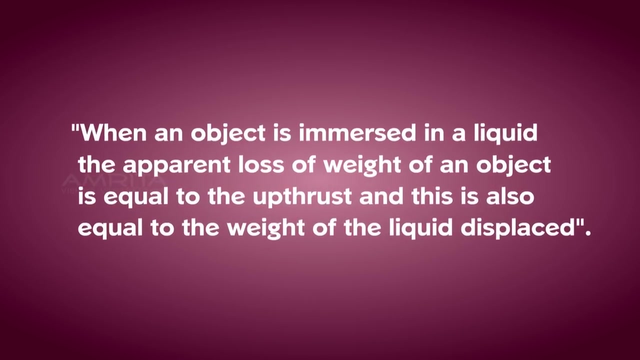 is equal to the weight of water displaced by it. This is better answered using the law of buoyancy, also known as the Archimedes principle, named after the Greek scientist who discovered it. Archimedes principle states That when an object is immersed in a liquid, the apparent loss of weight of an object is 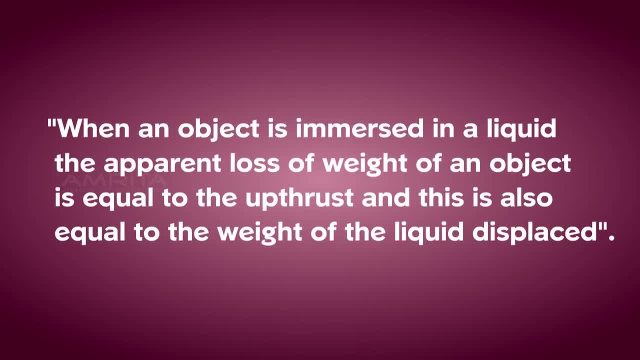 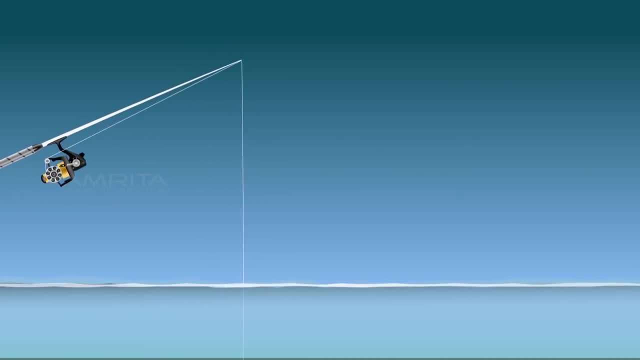 equal to the upthrust and this is also equal to the weight of the liquid displaced. We see the uses of this principle in our daily lives. Ever caught a fish with a fishing line? When pulling the line, you would have felt the weight of the fish in water is lighter than when the fish has surfaced. 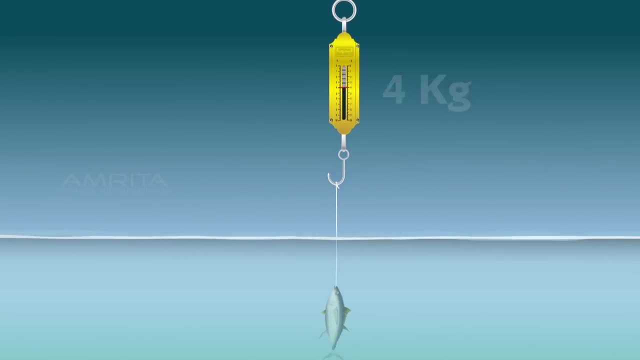 Say, the weight of the fish in water is 4 kilos, Its approximate weight outside would be 5 kilos. Well, the water level too has come down. This difference in the volume of water level will equal the loss in weight of the fish. 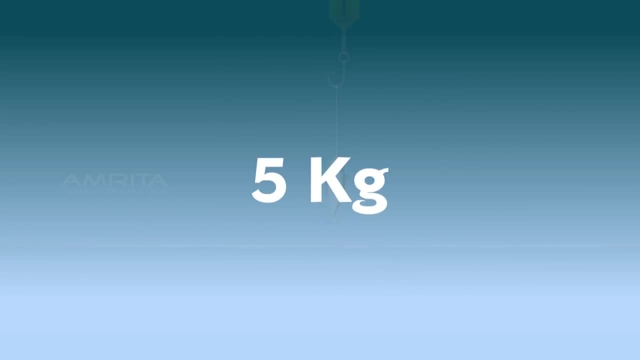 when in water. That is, the weight of the fish when outside, minus its weight when immersed in water, equals the loss in weight of the fish. So the loss in weight of the fish will equal the weight of the decreased water. This is because the upthrust or buoyant force is equal to the weight of the decreased amount. 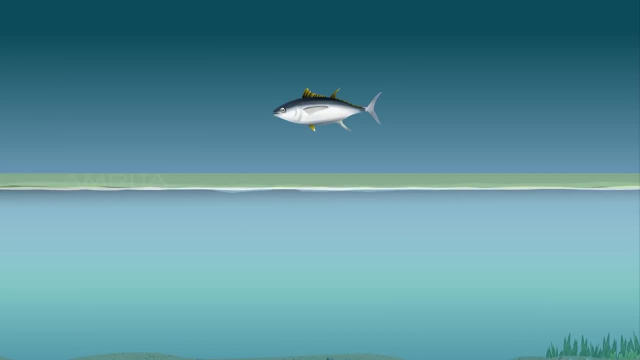 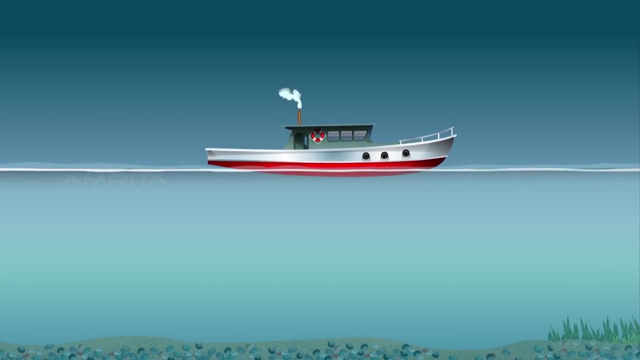 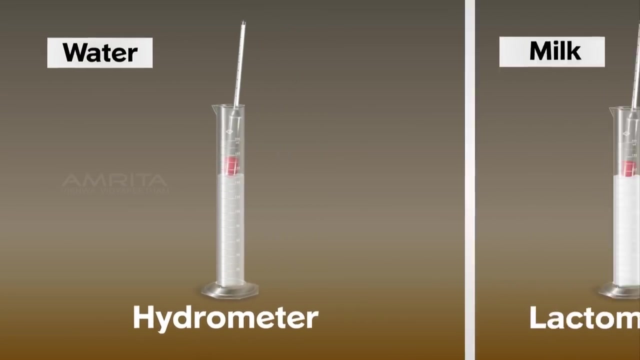 of water. Thus, Archimedes' principle is verified. Certain technologies today work based on the Archimedes' principle. To name a few, the designing of ships and submarines. hydrometer is used to find the specific gravity of liquid, and lactometers used to determine purity of milk. 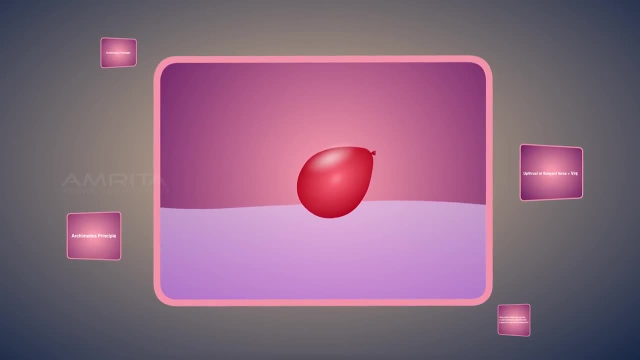 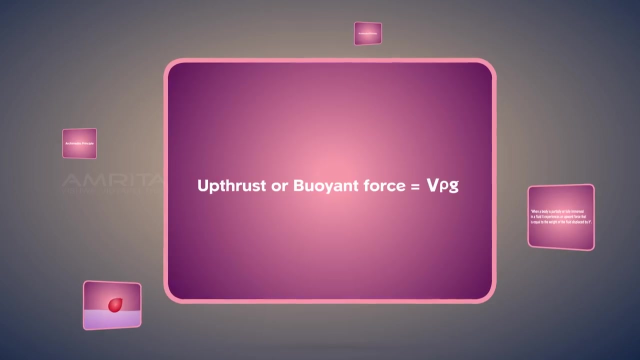 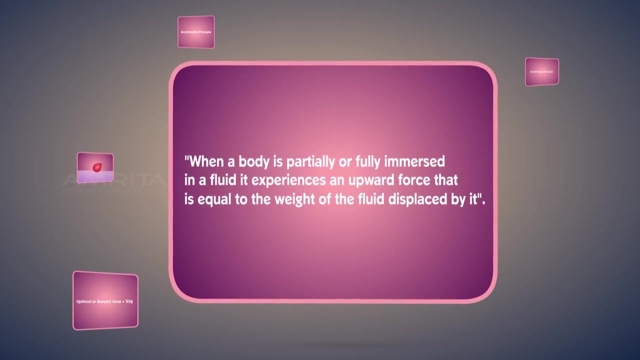 Things to Remember. The upward force exerted by a fluid is called upthrust or buoyant force. Upthrust or buoyant force equals v? rho g. Archimedes' principle states that when a body is partially or fully immersed in a fluid,